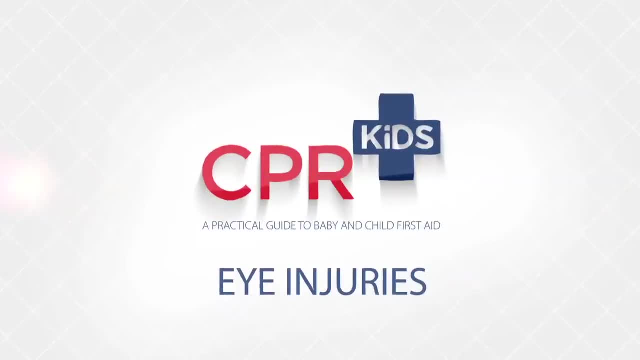 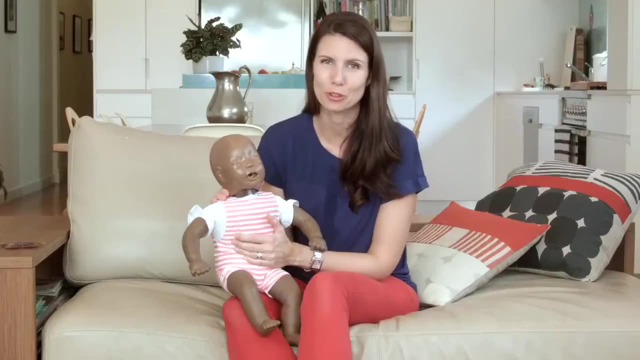 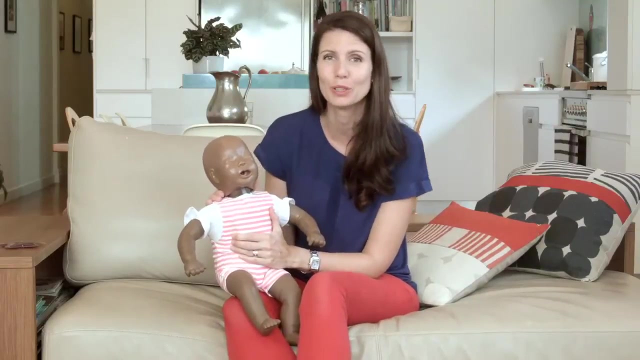 In this video we're talking about eye injuries, and these are very, very common in children, Often when they're at the playground in the sand pit and somebody else throws a fistful of sand into their eyes, or maybe a sibling comes along and has a little poke or a toy. 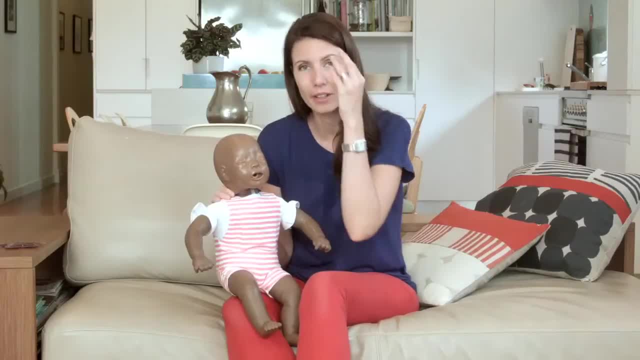 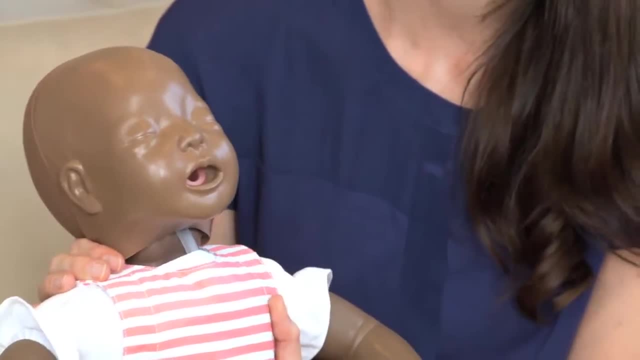 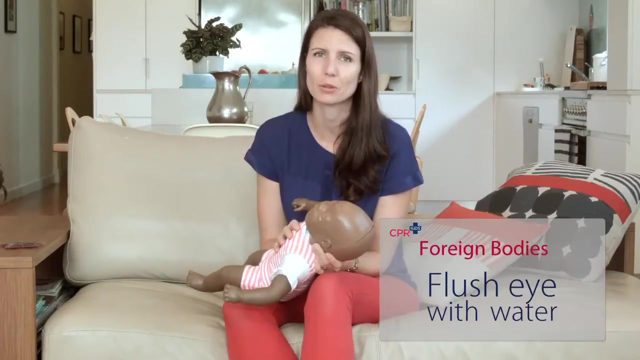 anything really. they can often end up with either a foreign body in their eye or even a scratch to the eye itself. Now, especially when it's a foreign body in the eye, we need to flush their eye with lots and lots of water, and this can be incredibly difficult in a 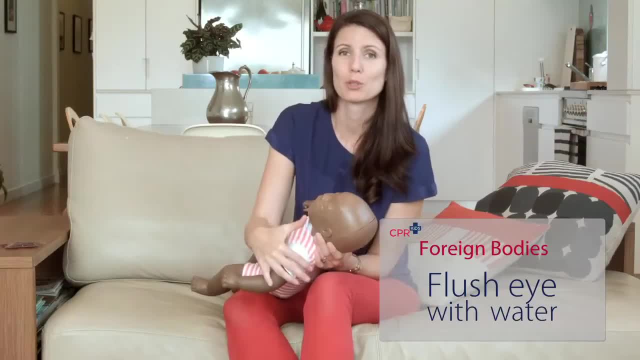 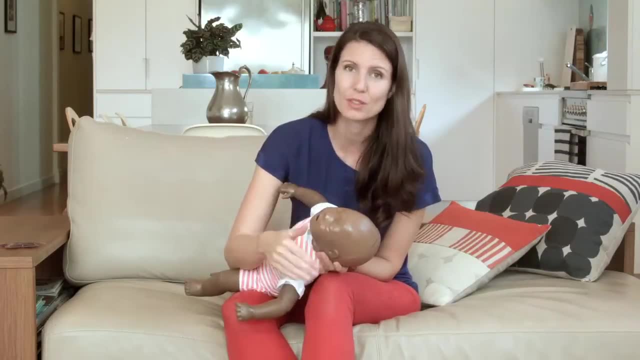 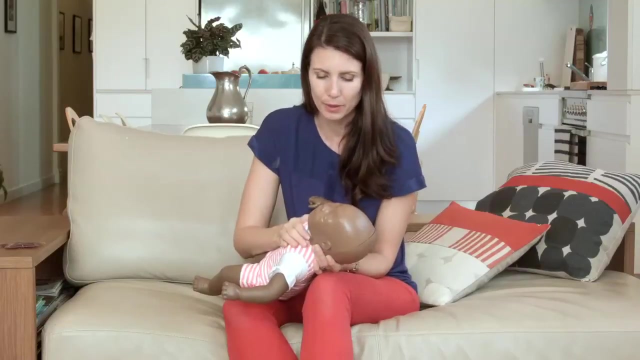 child. It is very, very hard to be able to pin down or restrain your child. hold their eye open, flush lots and lots of water through it. It can be really, really difficult and it's really traumatising for both the child and you. 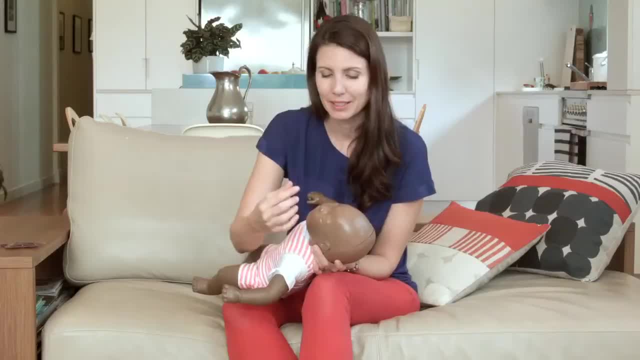 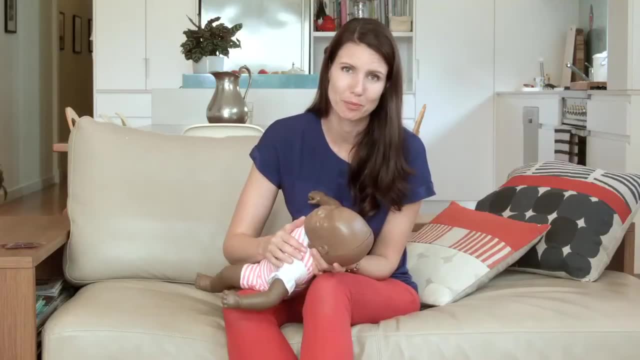 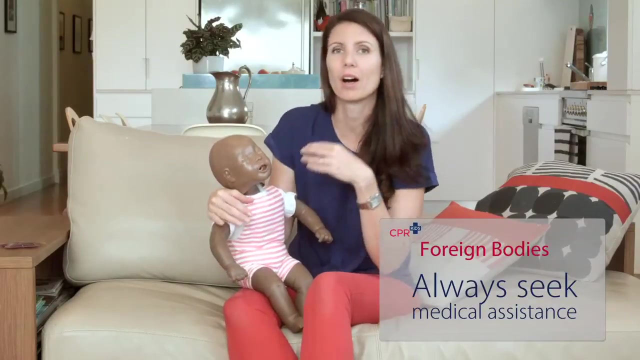 So if your child is not cooperating, if you are having too much difficulty being able to open their eye and flush that with water, you need to get medical help. So off to the GP or the hospital. they will be able to help hold your child open up the eye and flush that. 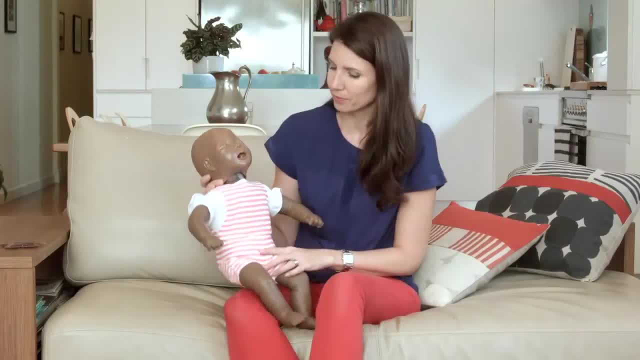 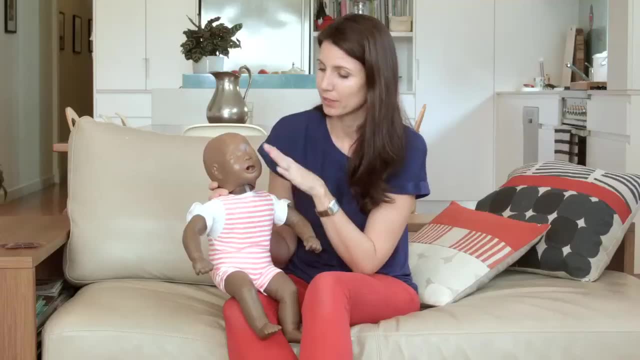 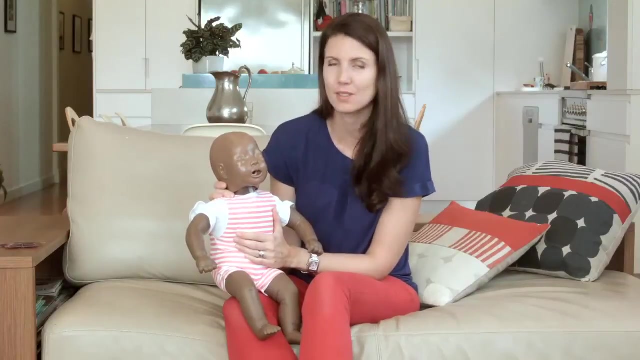 with water to try and get the object out, Even after. if you are successful flushing that out and the child is still complaining that there's something in there, then you need to get medical help. If you are not super conservative, we Тем to help with the care if youのre in need. 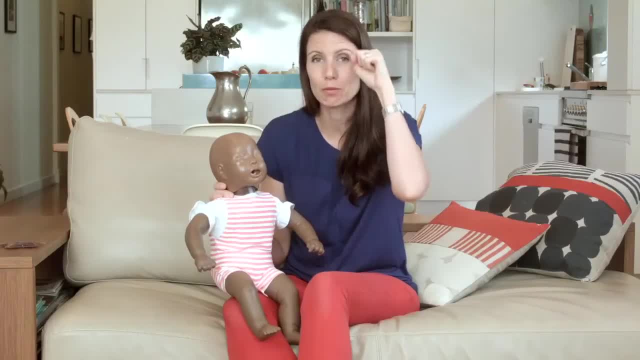 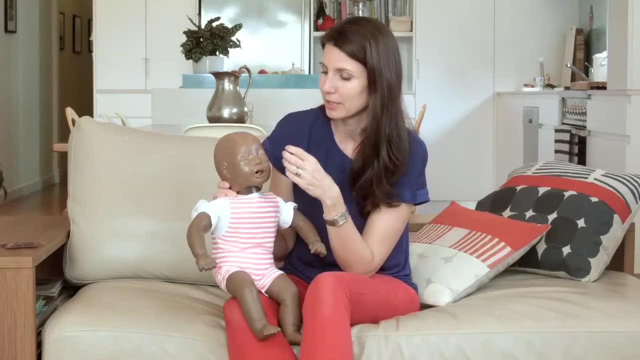 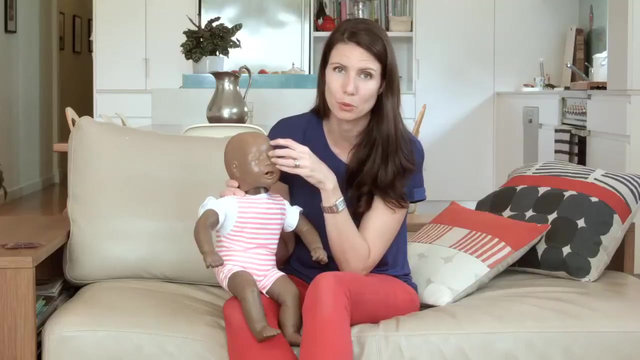 you. Transporting your child to see his doctor can get difficult because they really want to rub the eye, and rubbing música can make it so much worse, especially if they got a little piece of bark, stick or sand, That rubbing action can scratch their eye quite. 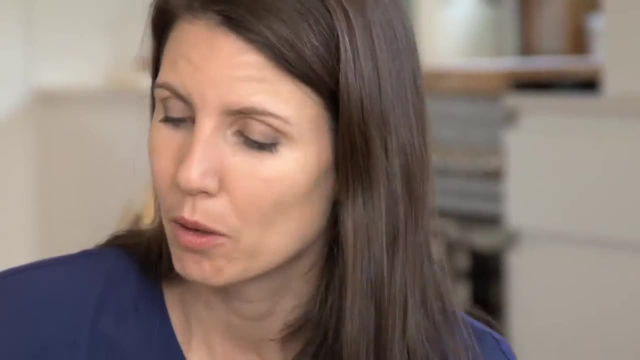 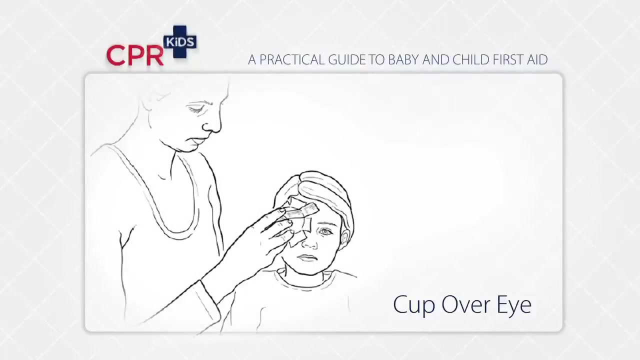 badly, so we need to take action in order to prevent them from doing that. If we put, that will cause pressure, So we need to put something on that's not pressing on the eye If we get a paper or a styrofoam cup.